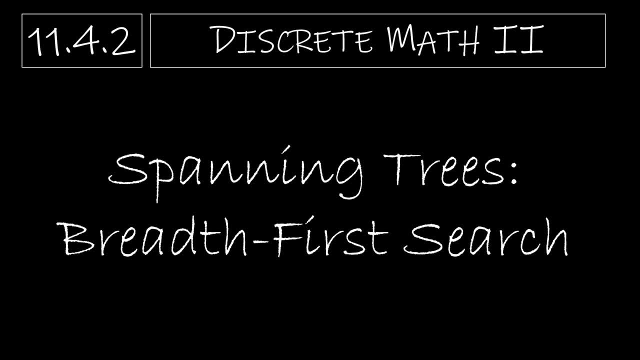 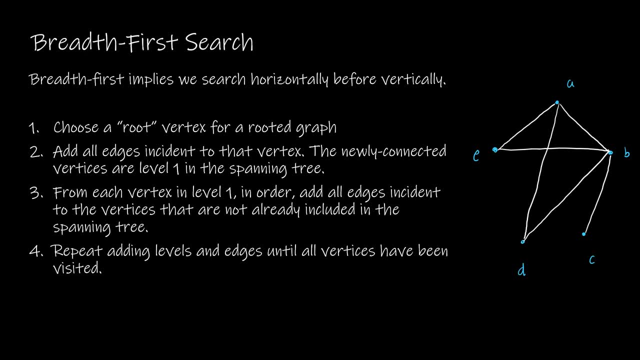 In this video, we're going to take a look at how to create a spanning tree using a breadth-first search. So how will a breadth-first search differ from a depth-first search? Well, if you'll recall, on our last video we started with a root node and then we chose the next vertex and went as far as 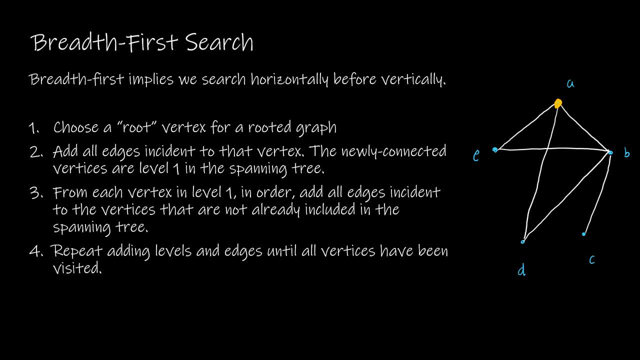 we could go with that particular vertex And in this case for a breadth-first search. instead we are still going to add whatever our root node is going to be, but then we're going to add all edges incident to that vertex. So in this case I would add AE and AB, I would add those edges. so I'm 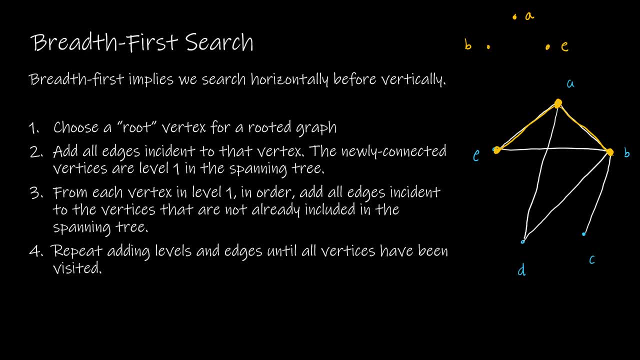 going to add B and E to my directed rooted graph, which is, of course, how we're going to look at the spanning subgraph. So, starting at A, I would connect to B and E. Now, the important thing here is that we have to have some order, So you can go with alphabetical order or you can have whatever other order you choose. 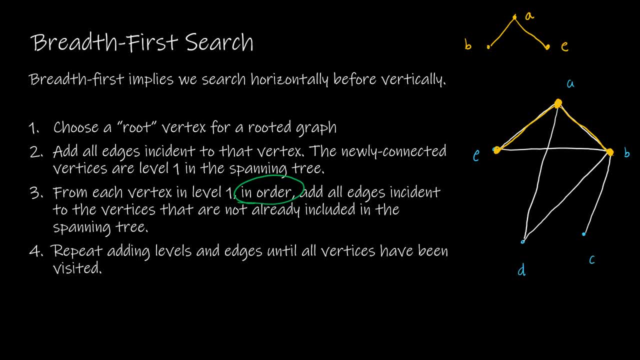 but the reason that this is important is I'm going to actually add an edge that wasn't originally in our graph to demonstrate how the algorithm might fail. So, if I don't have an order, as we can see E connects to C and B connects to C, and those are my two vertices that I'm dealing with. 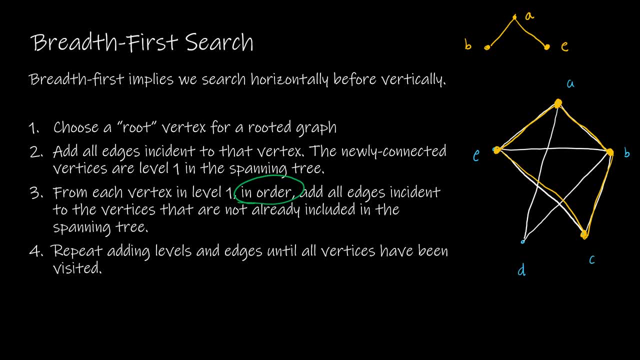 So the question is: according to the algorithm, should B be the one that connects to C or should E? So if you have an order and say I'm going to use alphabetical order, then it's clear to the algorithm that we're going to be starting from B. So from B I'm going to connect to both C and D. 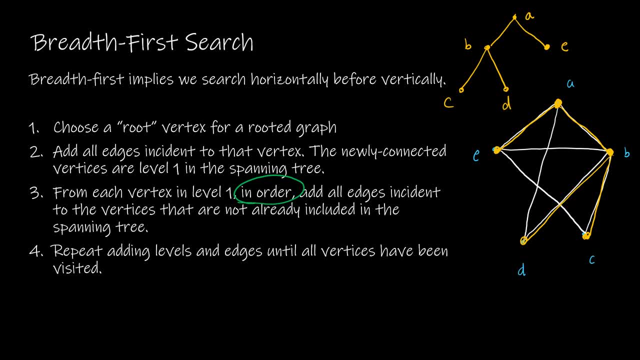 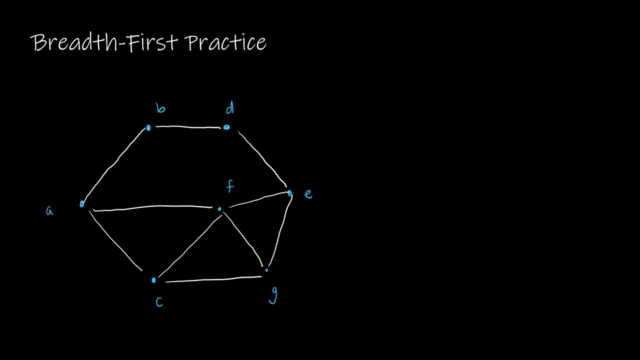 And now I've reached each of the vertices in my spanning tree, Whereas if there was no order, it would not be clear: should E connect to C or should B connect to C? This question may look familiar, as we did it in our last video, but we were using a depth first search rather than a breadth first. 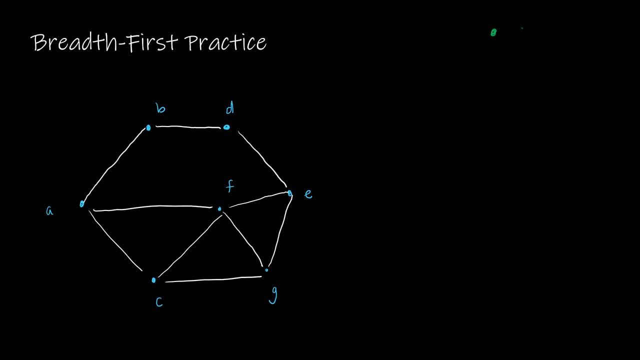 search. So we're going to go ahead and do the exact same example, just using a different algorithm. So this algorithm says we're going to connect to C and B and we're going to connect to C and D. So we're going to start at A and we're going to connect all of the vertices that are adjacent to A. So 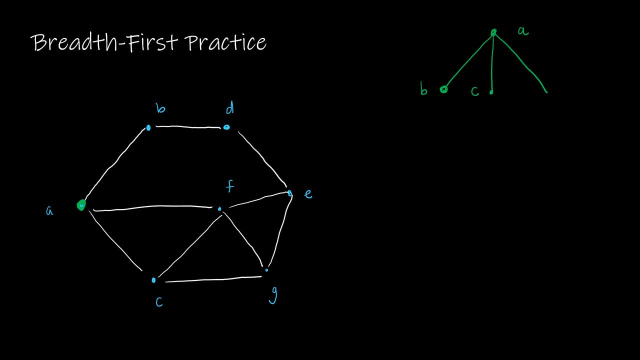 that would be B and C and F, And I am going to use alphabetical order as my order. So I've now connected B and F and C. Again, order is important. Order says now, starting from B, what can you connect to? So I'm going to connect to D. 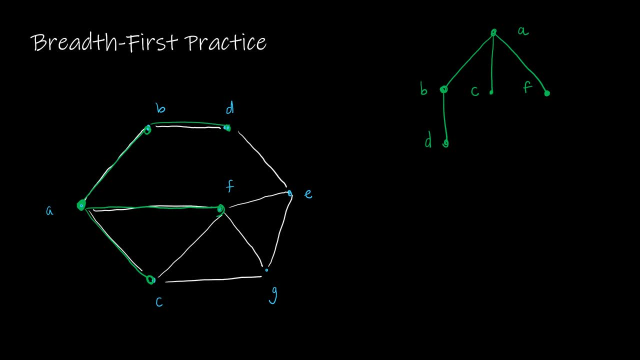 And I'm not going to connect to B, So I'm going to connect to D And I'm not going to connect to B, So I'm going to continue from D. I'm now going to move over to C, So what can I connect to from C? 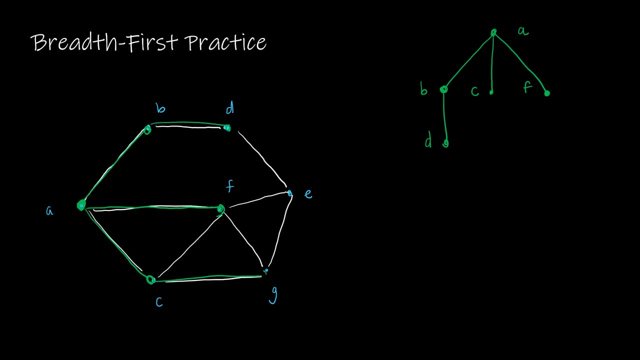 Well, obviously I can connect to F, but I'm already there, So I'm going to connect to G. So from C I'm going to connect to G And from F I'm going to connect to E. So that is what my breadth first. 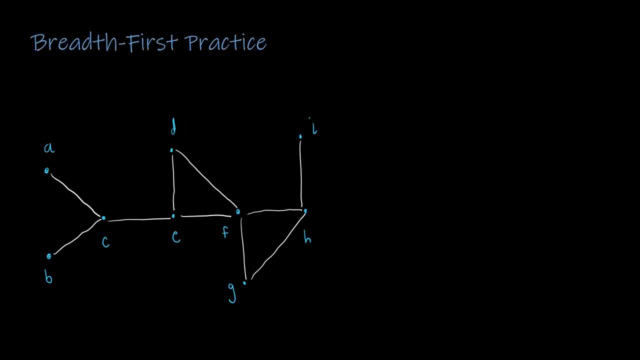 search spanning tree would look like: Here's one last practice for you to try on your own Using a breadth: first search. When you are ready, press play to see how you did So. again, I will start with A, And where you start is sort of arbitrary, But we'll start with. 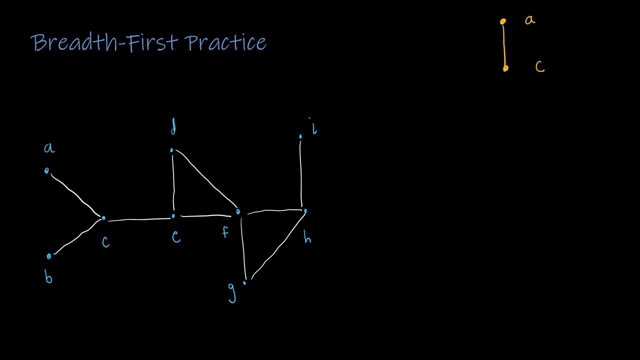 A. A connects only to one other vertex, which is C, So now I've visited both A and C. C connects to two vertices, B and E, And so now I've connected both of them to one other vertex, which is B, And so now I've connected them to one other vertex, B and C. 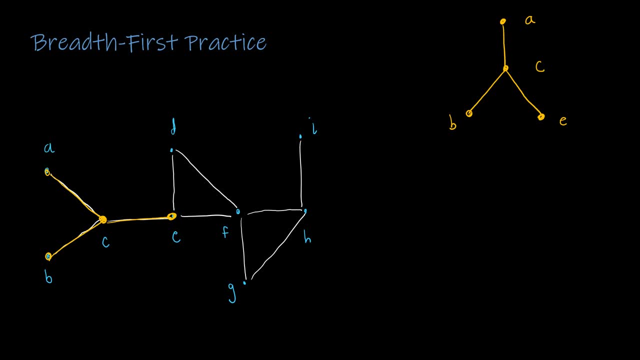 I've visited both B and E. B doesn't have any other vertices adjacent to it, so E is going to connect to both D and F. Again, I'm going to use alphabetical order as my guide, so from D I can connect only to F, which we've already visited. so I'm now going to branch off of F to visit both G.